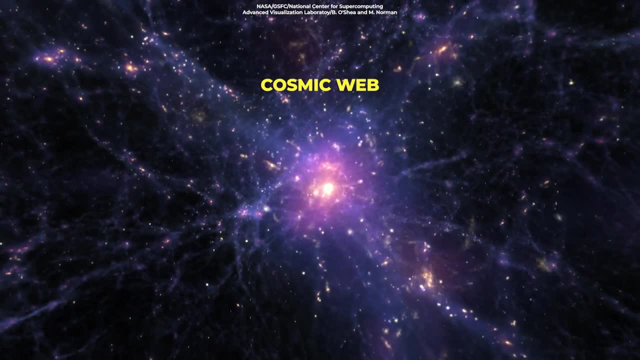 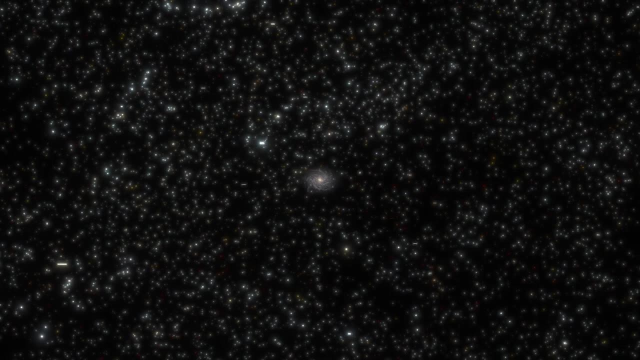 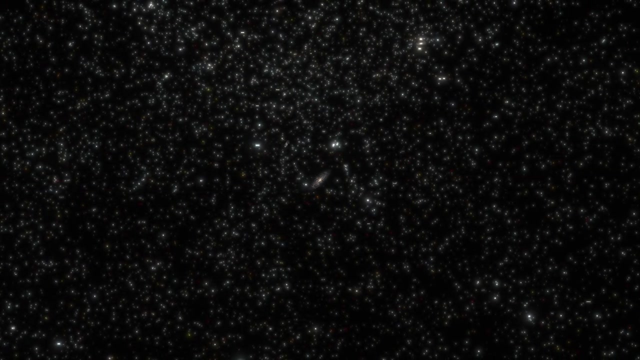 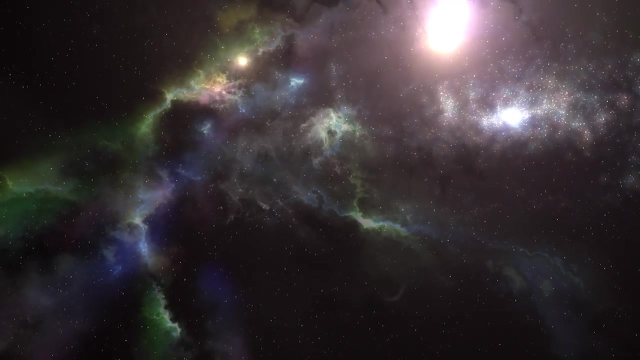 creating a massive foam-like structure known as the Cosmos. Before 1989,, it was believed the galaxy clusters that had a dynamic equilibrium were the most prominent structures in existence and that they were distributed more or less uniformly throughout the universe in every direction. However, since the early 1980s, more and more massive structures 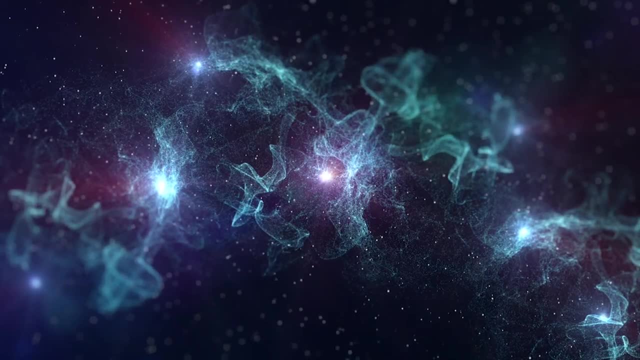 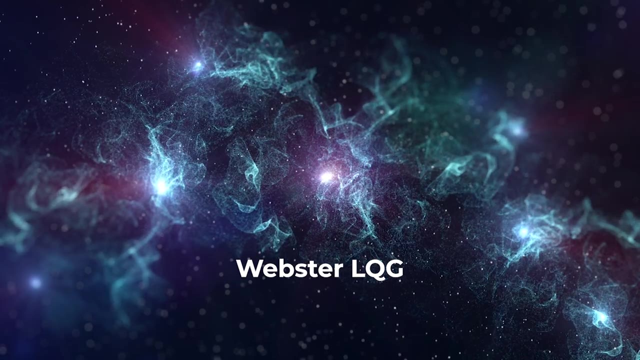 had been discovered. In 1983, Adrian Webster identified the Webster LQG, a large quasi-gaussian structure with a diameter of 1.6 times the size of the Earth. It was a large group consisting of five quasars. A quasar is an astronomical object of very high luminosity. 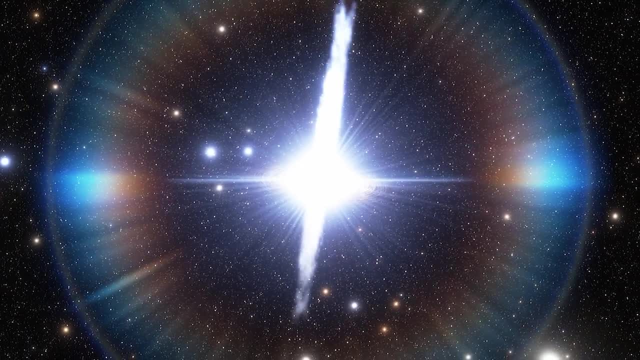 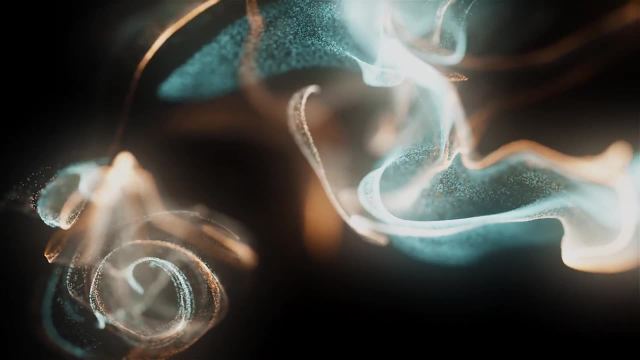 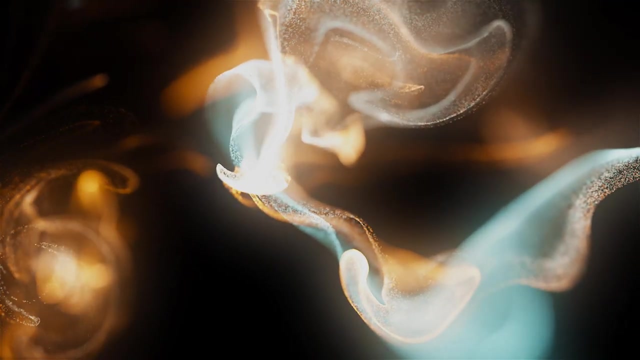 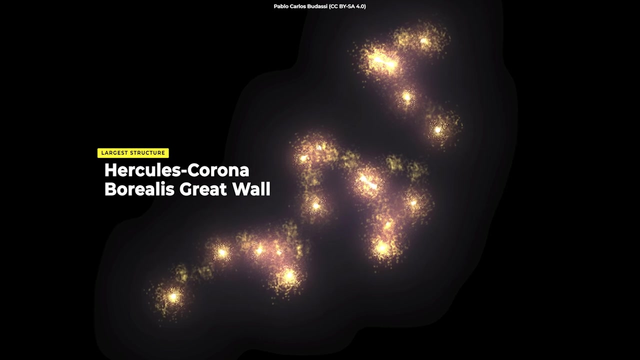 found in the centers of some galaxies and powered by gas spiraling at high velocity into a vast black hole. This discovery was the first identification of a large-scale structure and has expanded the information about the known grouping of matter in the universe. Currently, the largest structure in the universe is Hercules-Corona-Borealis Great Wall. 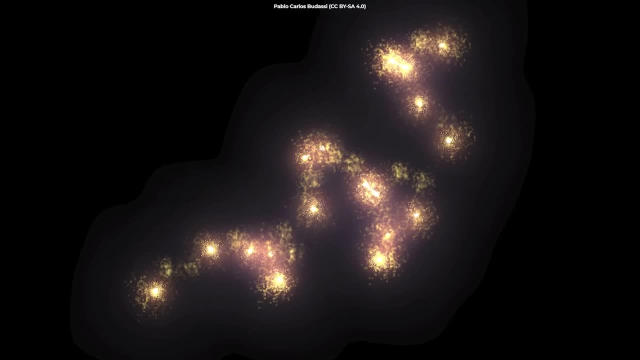 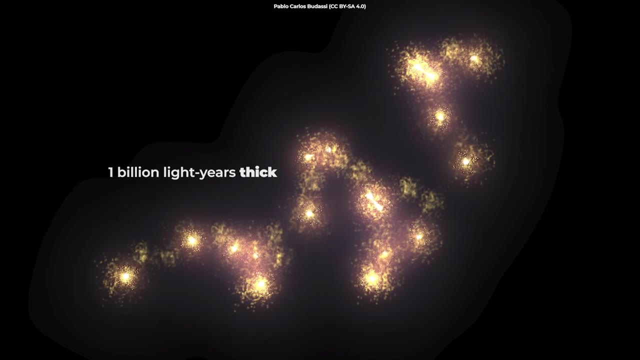 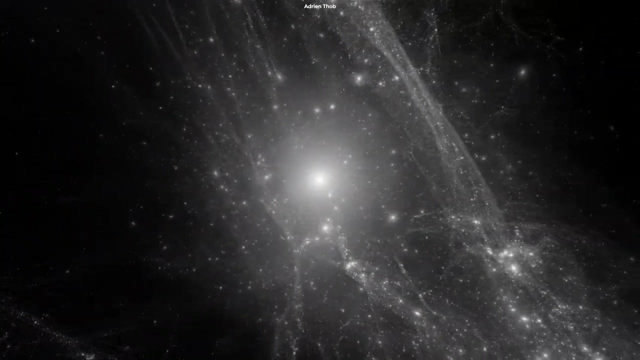 which was discovered in November 2013.. It is approximately 10 billion light-years long, 7.2 billion light-years wide and almost 1 billion light-years thick. Groups of galaxies are not randomly distributed throughout the universe, but are grouped into gravitationally bound clusters. 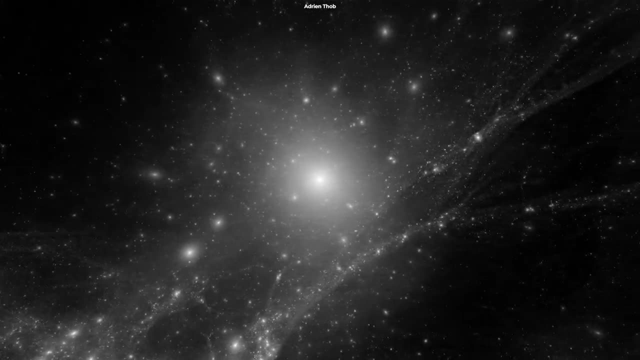 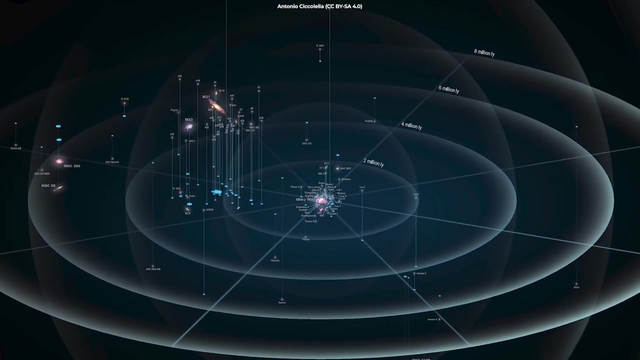 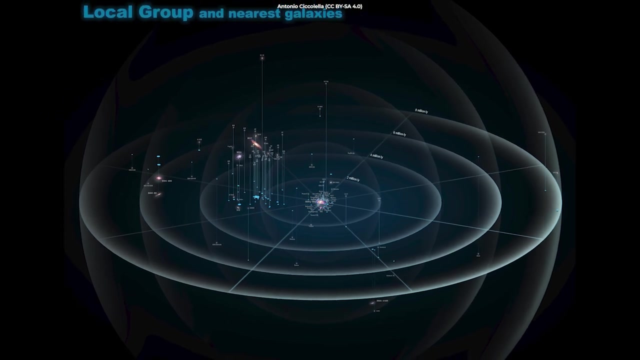 These clusters are called clusters of galaxies. These clusters are described as rich or poor, depending on how many galaxies they contain. Poor clusters are called groups, and our Milky Way is part of a poor cluster called the Local Group. The Local Group comprises more than 50 galaxies, including the Dwarf Galaxies. 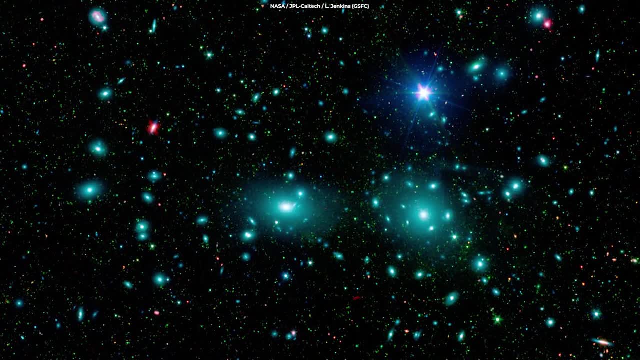 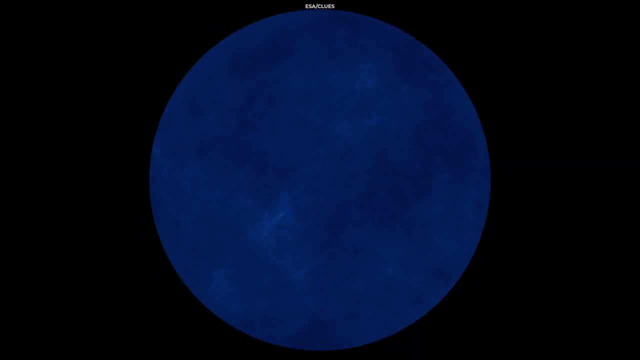 Rich clusters contain over 1,000 galaxies, and an example is the Coma Cluster that has about 10,000 galaxies. The clusters are the largest clusters of galaxies in the universe. These clusters are then grouped into superclusters consisting of around a dozen clusters. 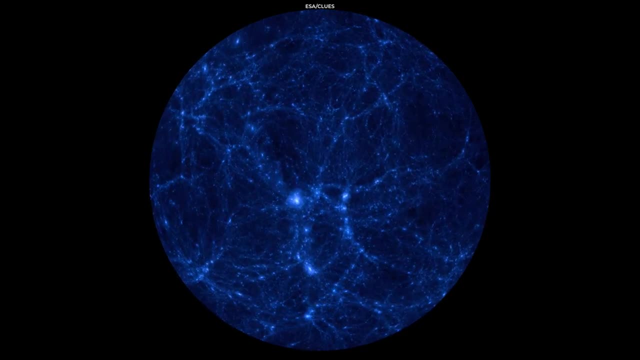 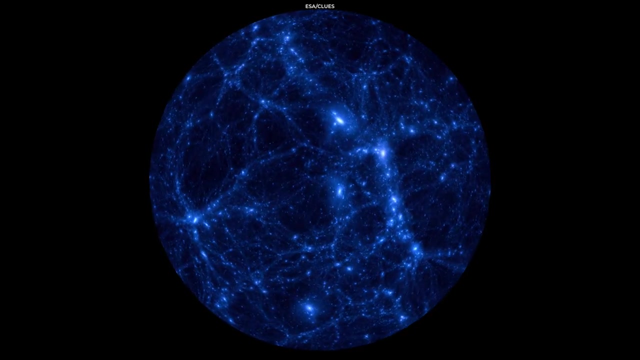 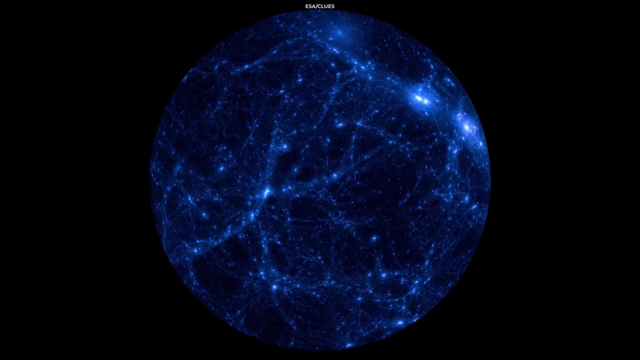 each with a mass of about 10 trillion to 100 trillion solar masses. Superclusters are the largest known systems of galaxies. The largest superclusters can spread over several million light-years of space. That is how massive the superclusters are. There are two large-scale clusters of particular importance in the massive universe.